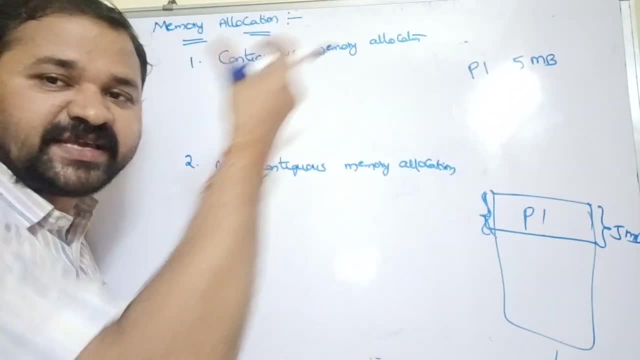 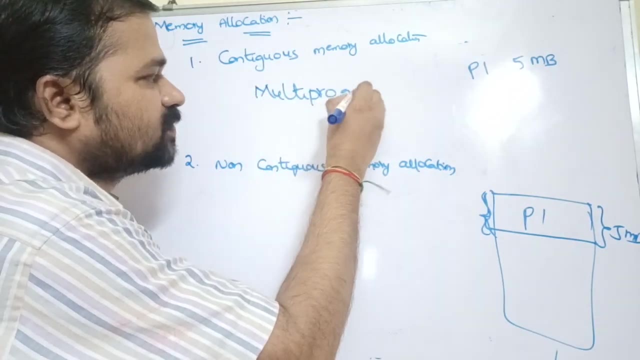 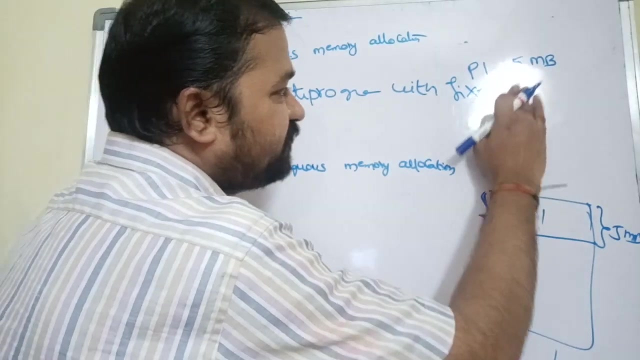 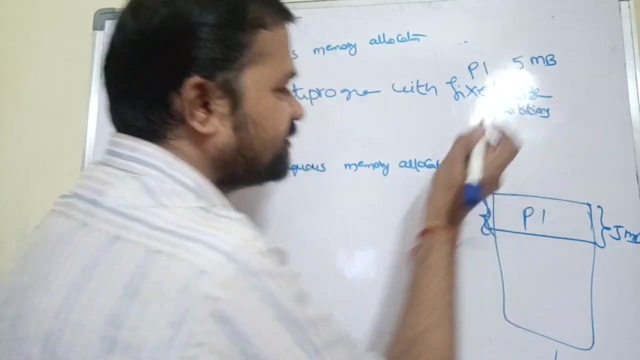 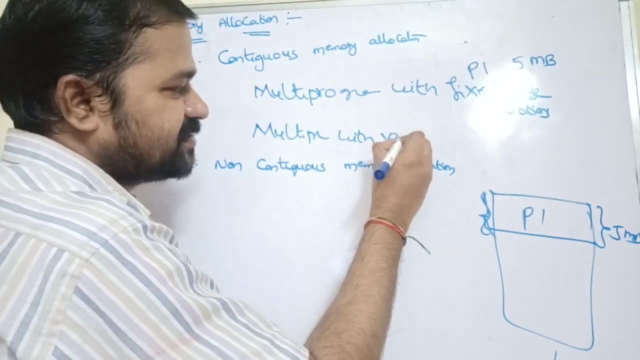 There are two approaches for implementing contiguous memory allocation. The first approach is multi-programming with fixed partitions, Multi-programming with fixed size partitions, Multi-programming with fixed size partitions, Whereas the second approach is multi-programming with variable size partitions, Multi-programming with variable size partitions. 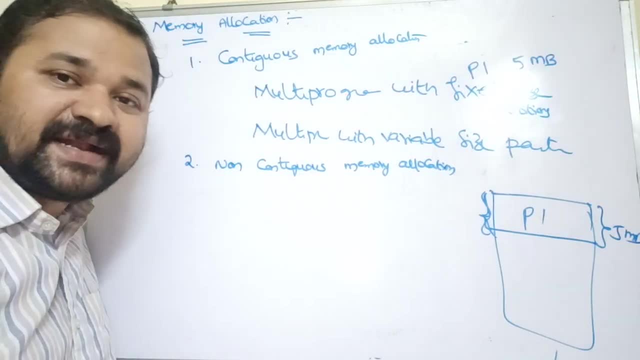 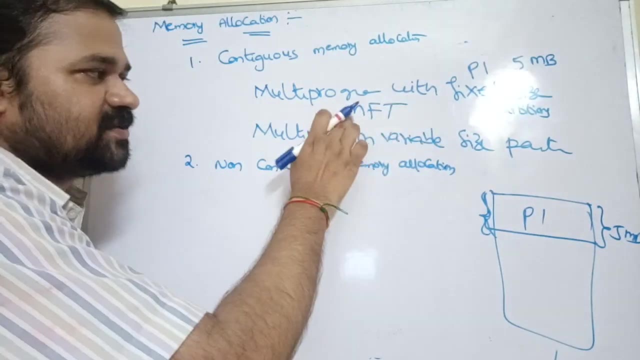 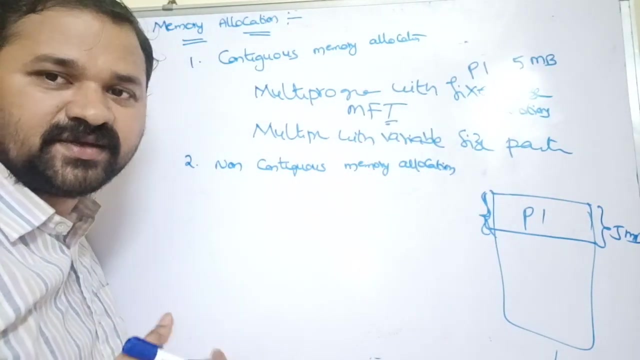 So what is the first approach? Multi-programming with fixed size partitions. In short, we can call as MFT. So M stands for multi-programming And v stands for variable size And f stands for fixed size, Whereas d stands for tasks. 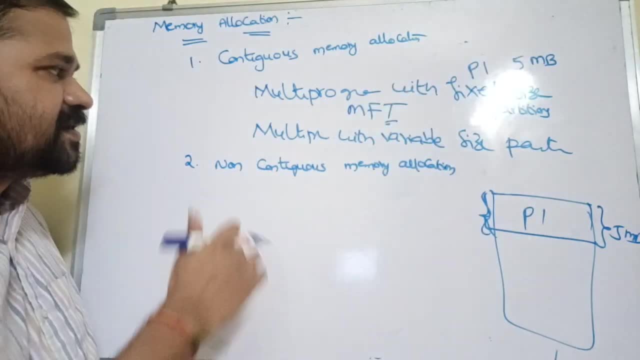 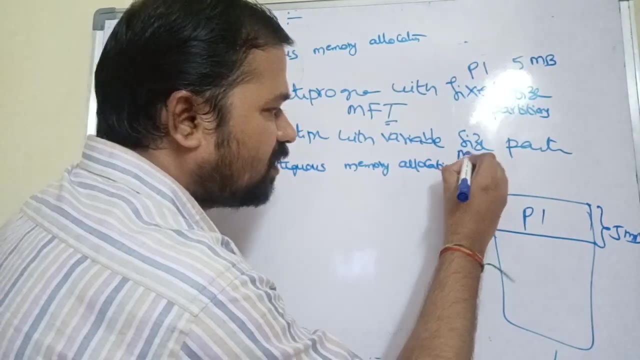 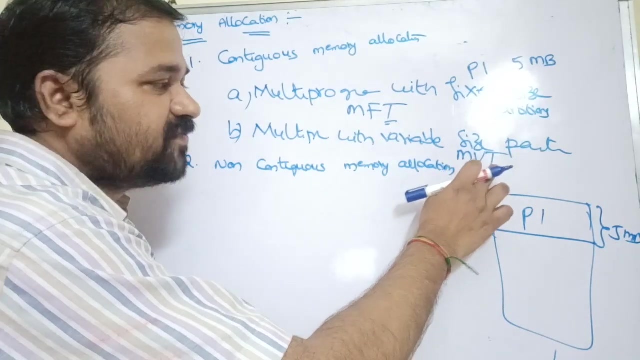 So tasks are nothing but some processes or some partitions. Whereas what is the second approach, Multi-programming with variable size partitions. So, in short, we can call as MVT. So M stands for multi-programming, V stands for variable size, whereas d stands for some tasks. 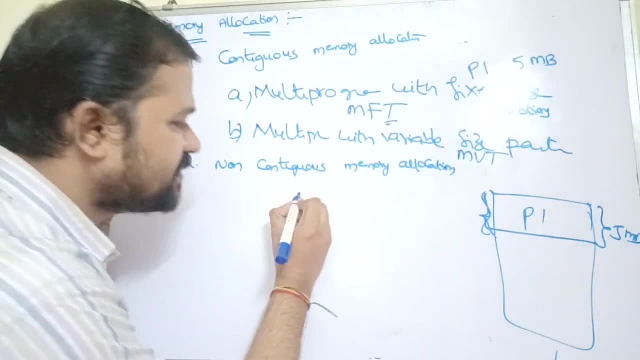 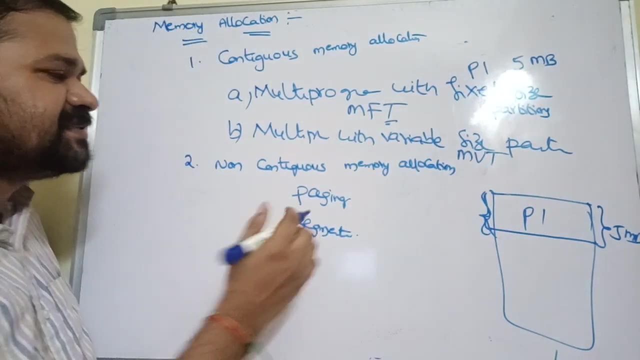 Okay, And the second approach is Non contiguous memory allocation. The best examples for non-contiguous memory locations are pacing and segmentation. So here, non-contiguous means whenever there is a free space, then we can store the process in that free space. 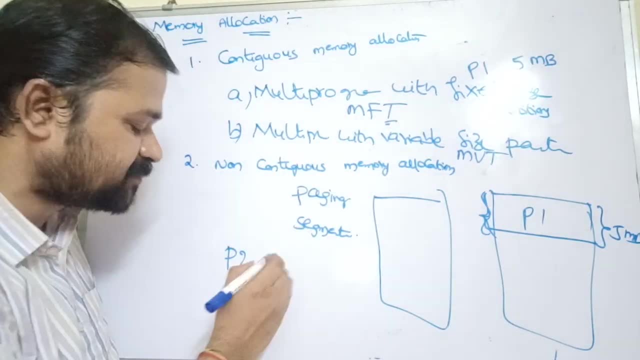 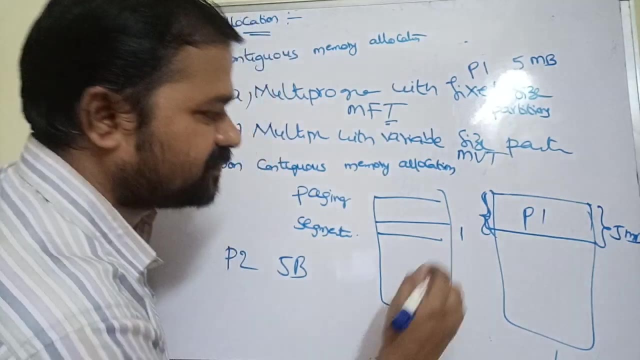 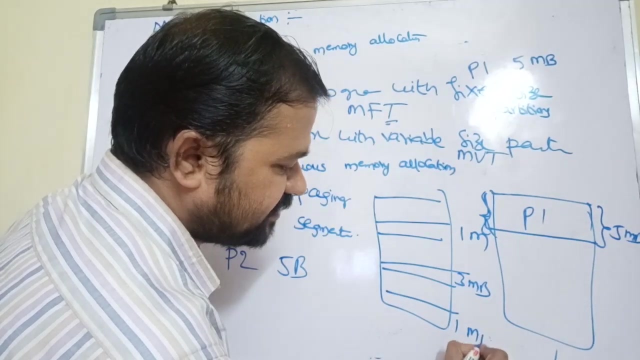 So let the size of let process name is P2, whereas the size of a process is 5 MB. So let we have 1 MB free space here. Let we have 3 MB free space here. Let we have 1 MB free space here. 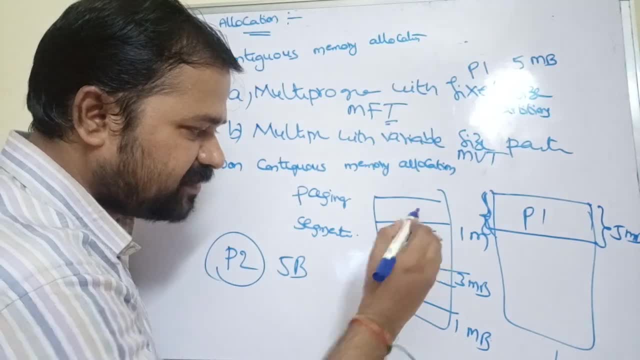 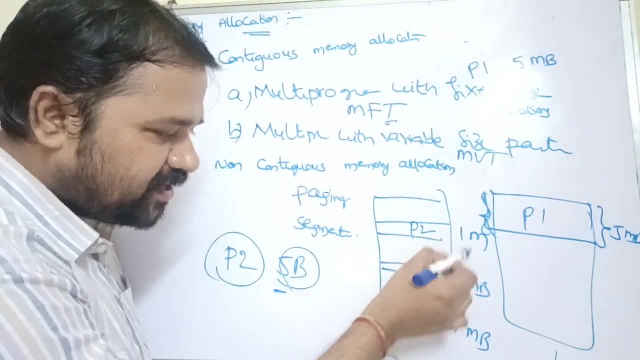 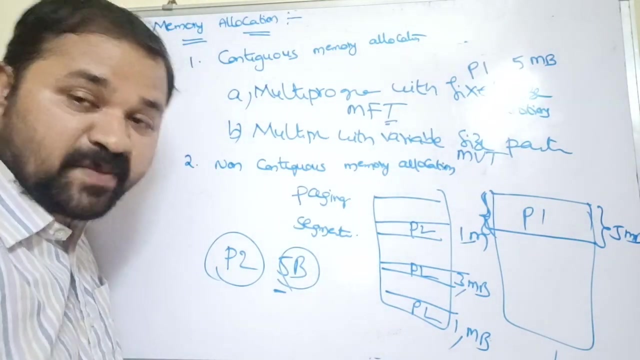 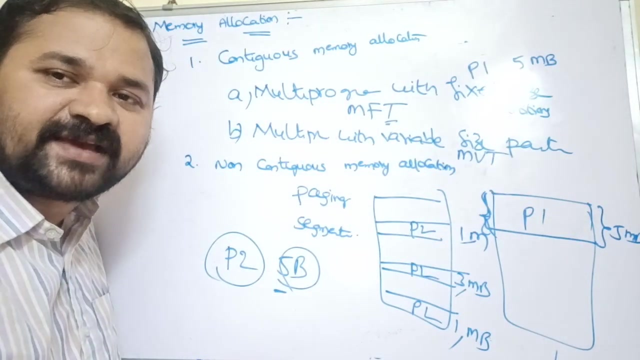 So we can store process P2 in this 1 MB in this partition, whereas in this partition. So what is the size of P2? 5 MB, So here. so this is 1 MB, So this is 1 plus 3, 4, 4 plus 1, 5.. So this is nothing but non-contiguous memory locations. So the memory locations need not be contiguous. So wherever there is a free space, then the operating system allocates that free space to the corresponding process. 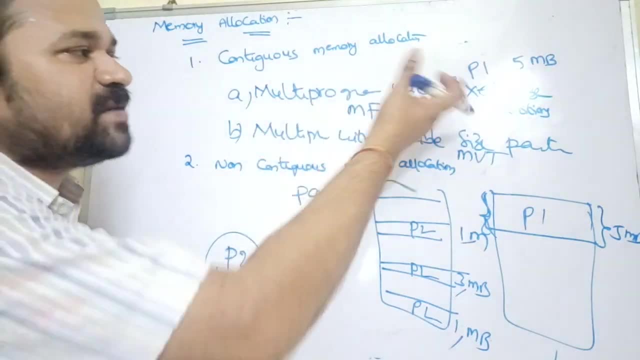 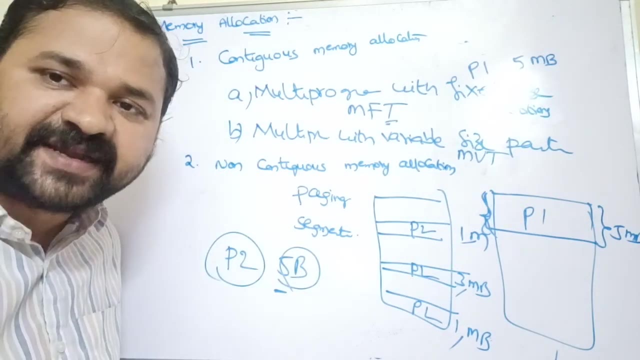 In the upcoming videos, we will discuss multi-programming with fixed size partitions, multi-programming with variable size partitions, pacing, as well as segmentation.